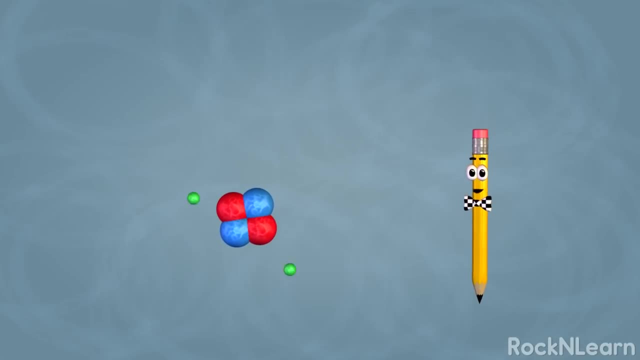 The tiny particles zipping around the outside of the nucleus are called electrons. In a real atom they move much faster. Electrons have energy. They have a negative charge- Protons positive, neutrons neutral, And outside the negative electrons reside. 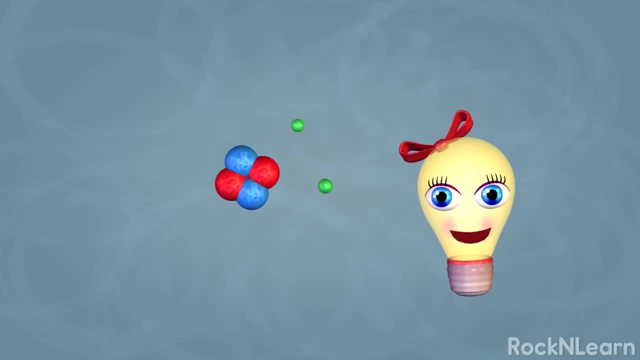 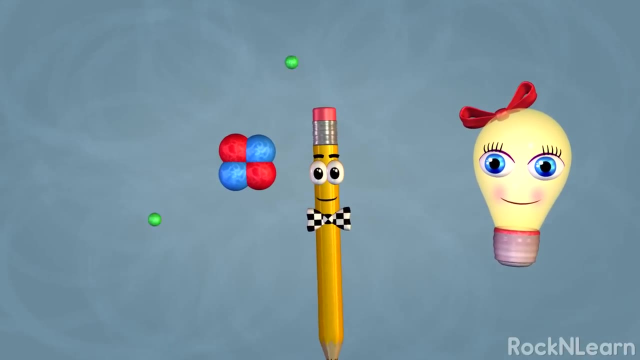 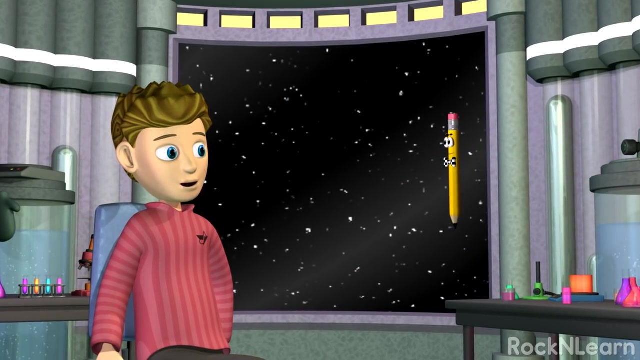 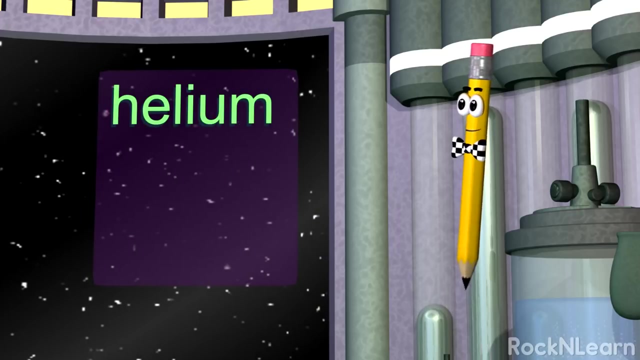 Protons, positive neutrons, neutral, And outside the negative electrons reside. So everything around me is made up of atoms. Does that mean I'm made of Kevin atoms? Oh, no, no, no. Some things like helium, oxygen and gold are made up of one kind of atom. 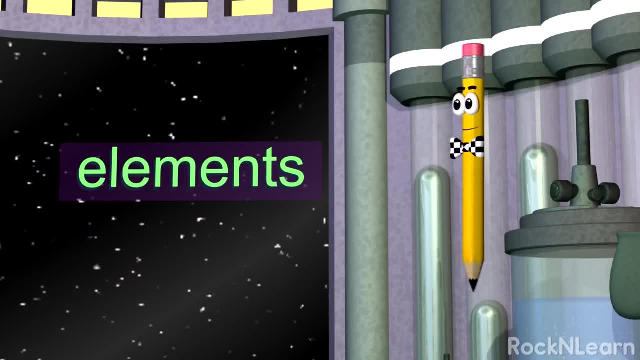 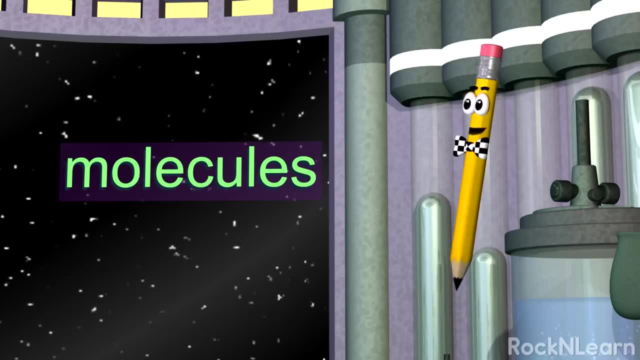 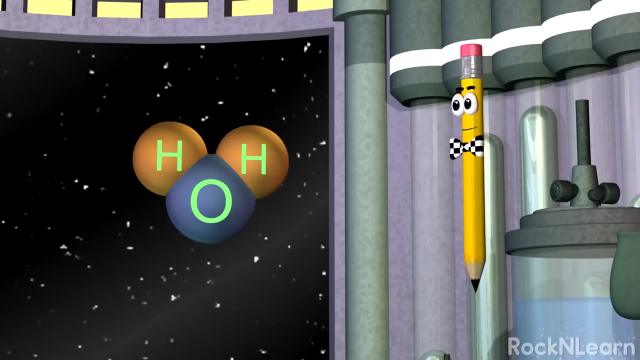 Things made of only one kind of atom are called elements, But sometimes different kinds of atoms will bond together to form molecules. For example, a water molecule is made up of two hydrogen atoms and one oxygen atom. Oh yeah, I've even heard people call water H2O. 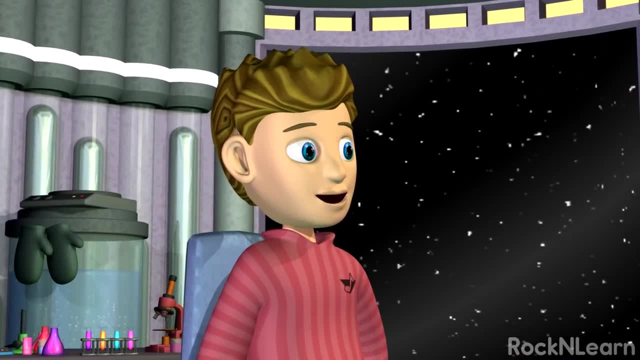 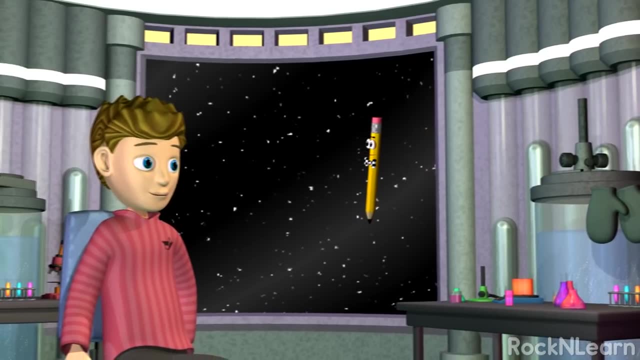 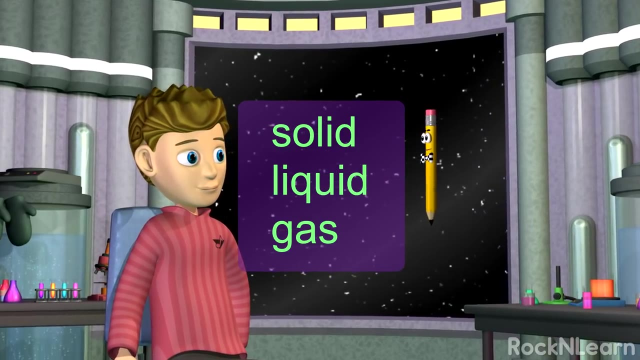 And water is completely different from hydrogen or oxygen by themselves. Now water, like all matter, can exist in different states. I've learned about states of matter: solid, liquid and gas. That's right, And matter can change states under certain conditions. 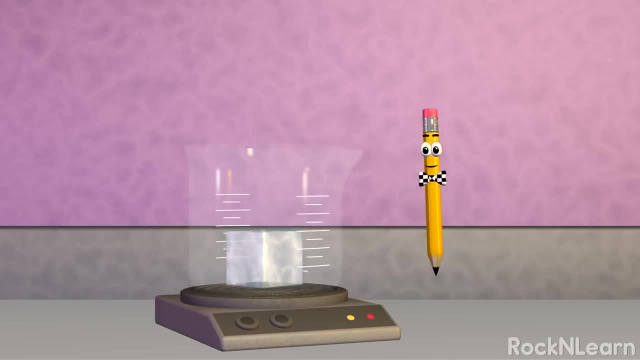 Let's consider water. In its solid form, water is called ice. But what happens when ice gets too warm to remain as ice? It melts. Oh, It changes state from solid to liquid at a certain temperature. The temperature at which it changes from solid to liquid is called the melting point. 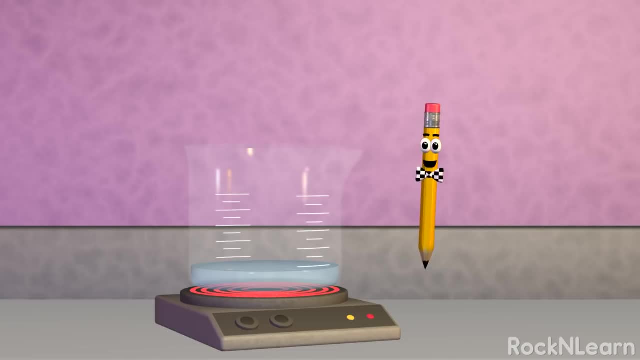 Now, if you heat the liquid water up to its boiling point, it will change to its air, That's right. It will change to its gas state, which we call water vapor or steam, Like in clouds, Correct? Each type of matter has its own boiling point and melting point. 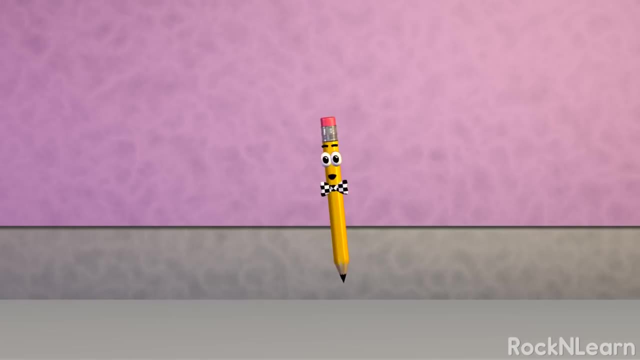 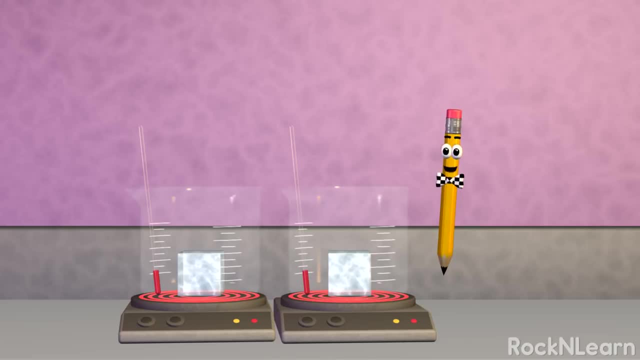 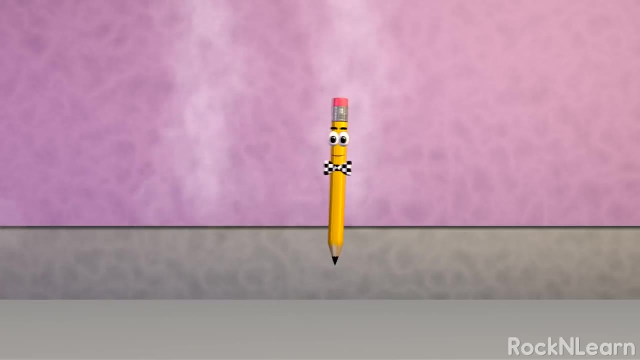 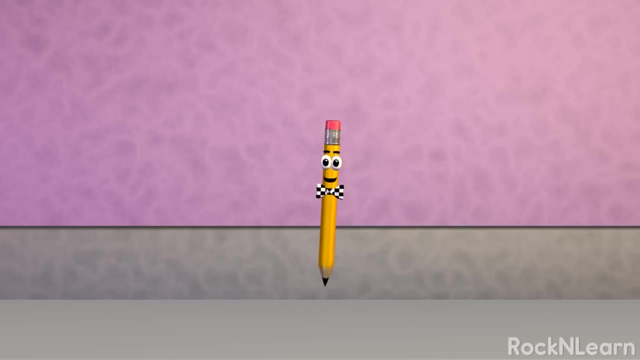 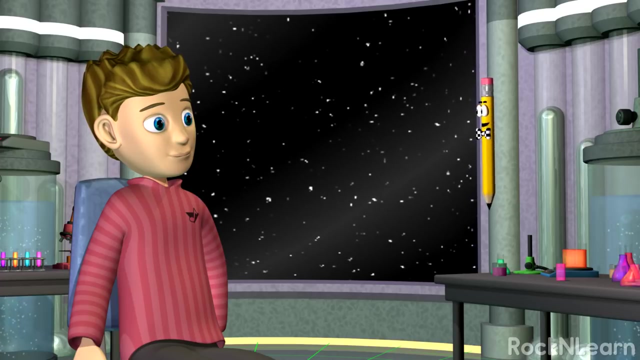 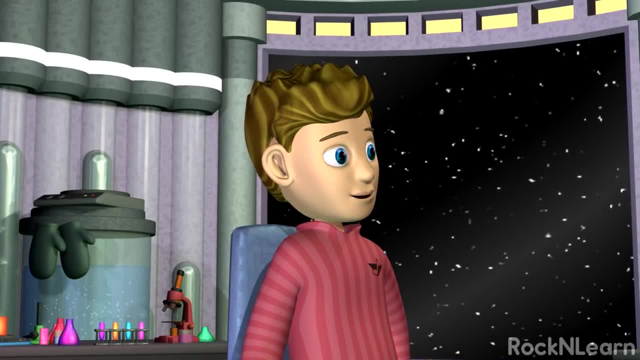 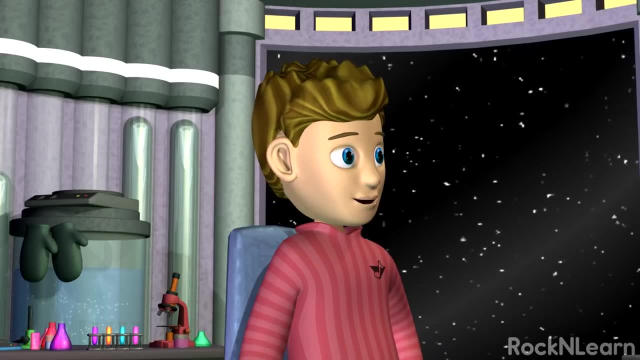 The point at which the liquid water turns to a solid is the freezing point. The melting point, boiling point and freezing point are only some of the properties of matter. Physical properties are things you can detect with your senses, Like cold day and it felt really chilly, But when I touched the door it didn't feel as cold. 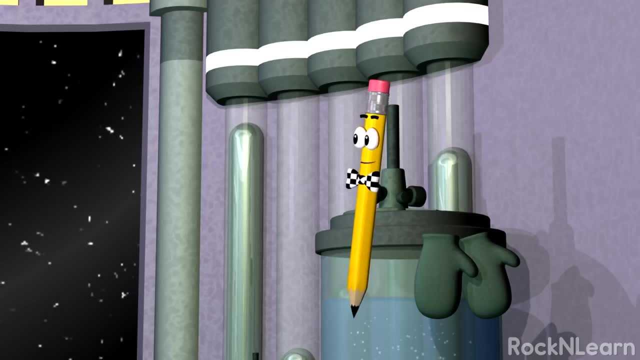 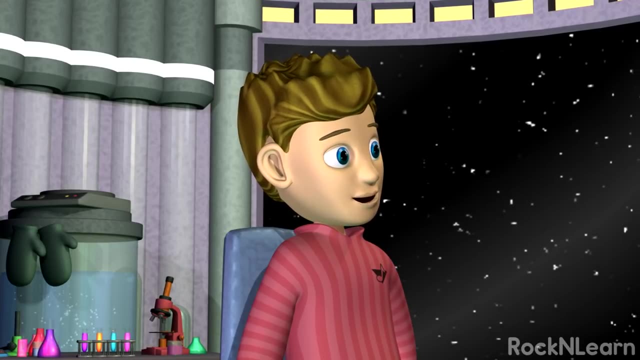 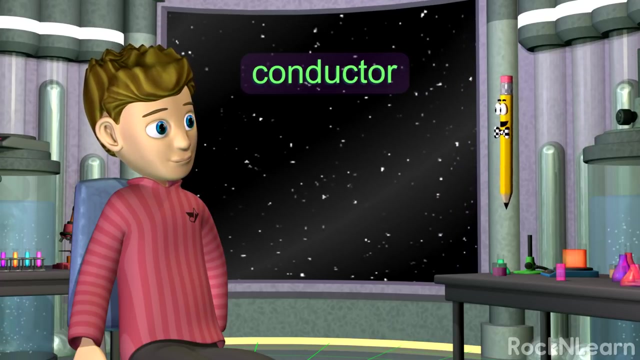 I'll bet the doorknob was metal and the door was wood. You're some kind of mind reader, So why did the metal feel colder? Aren't the doorknob and the door the same temperature? Yes, but metal is a better conductor than wood. Heat leaves your hand more quickly when you touch. 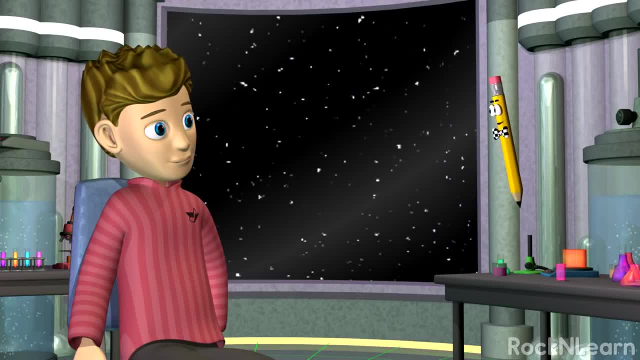 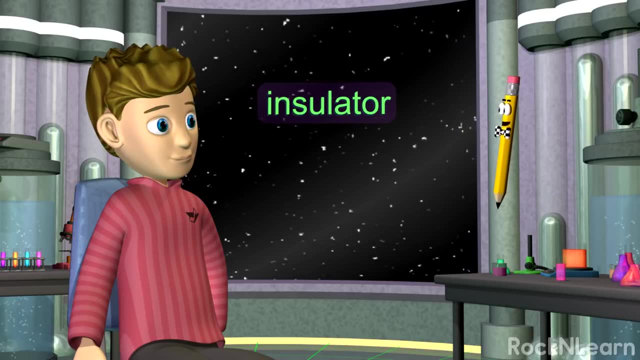 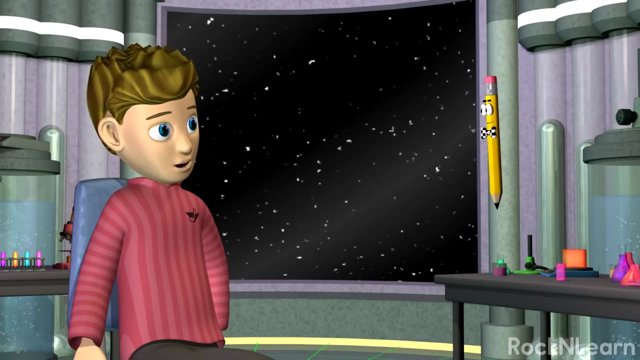 the doorknob. so the metal feels colder than the wood, even though they are the same temperature. Wood is a better insulator than metal. If you had on mittens, the metal would not feel as cold, because mittens are good insulators too. So that's another property of matter. 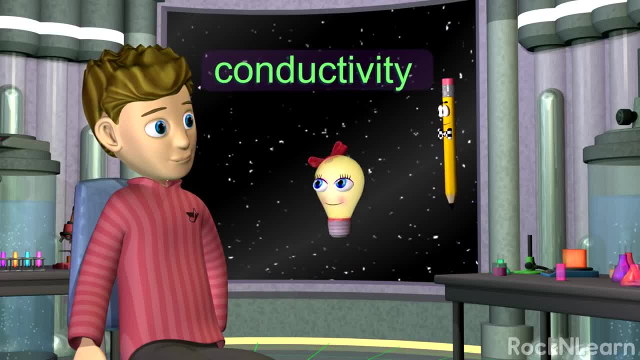 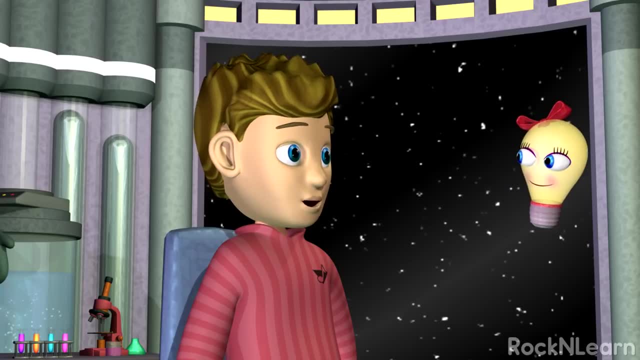 And it's called conductivity. Metals are also good conductors of electricity. I suppose you'd know about that, Lumina. Let's think about it. Let's think of some more properties of metals. Hmm, they tend to be shiny, especially if you polish them. 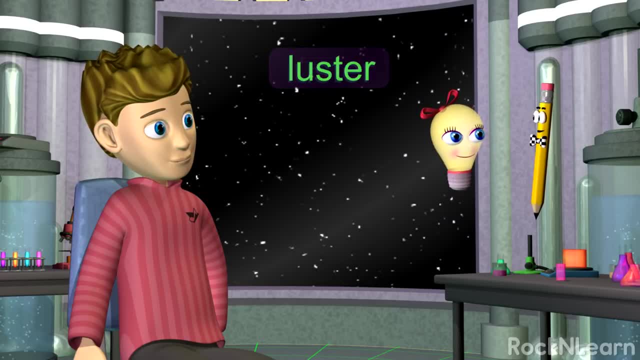 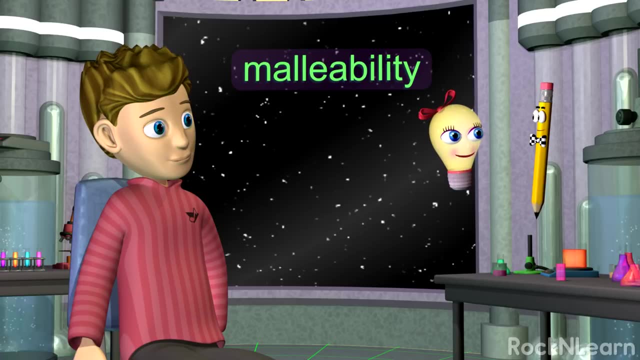 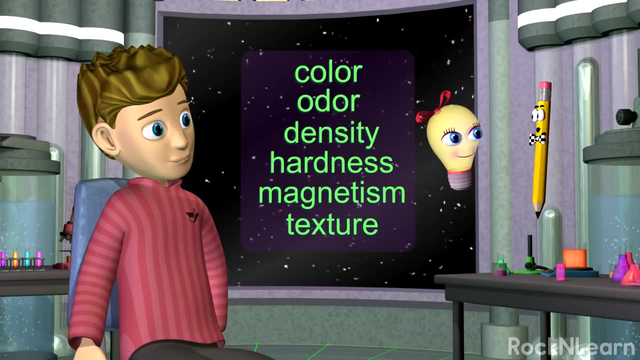 You're talking about luster. Another fun property of metals is malleability. Ooh, that means that metals can be bent and shaped into important things like wires. There are so many more properties of matter: Color, odor, density, hardness, magnetism and texture. 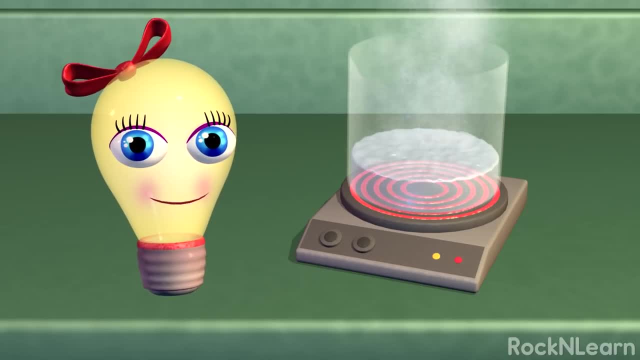 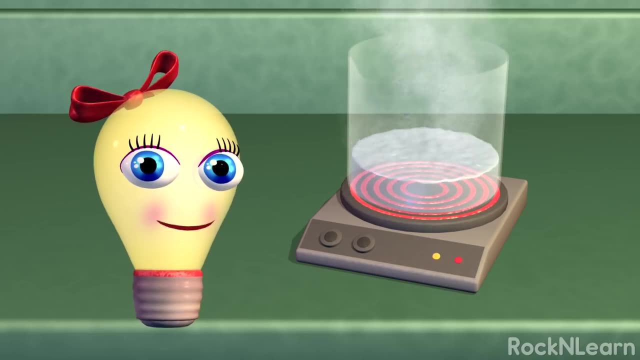 Just to name a few. What's this? Looks like you boys have been making some physical changes. Huh, What do you mean? This water boiling is a physical change of matter. Even though the state changes from liquid to gas, the molecules are still H2O, still water. 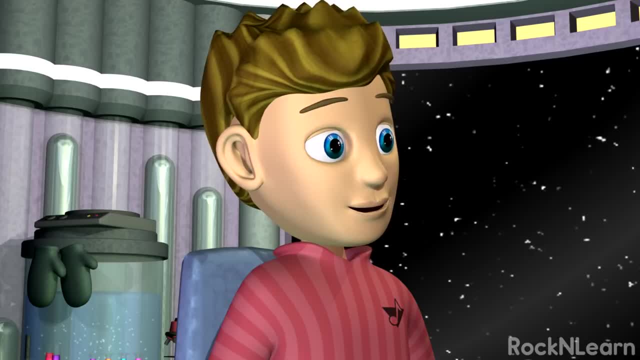 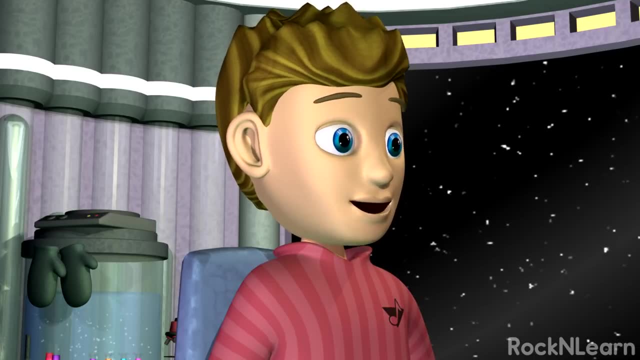 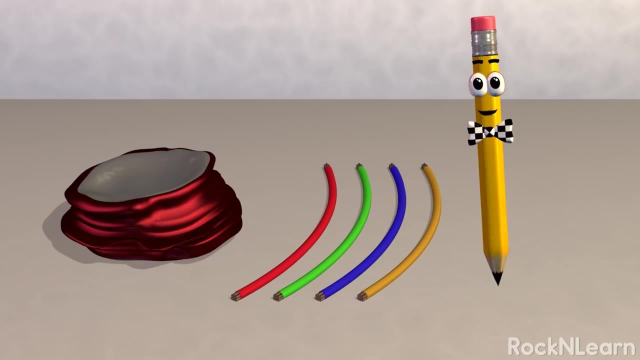 I get it. Physical changes don't change the chemical properties of matter. Like if I break a wooden pencil in half, both pieces are still made of water. Why don't we think of a different example? How about crushing a can? or forming metal into wires? 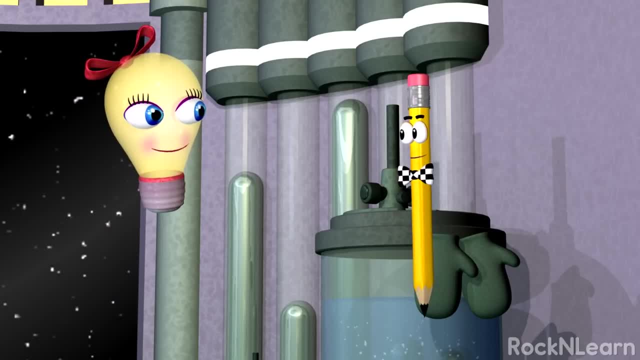 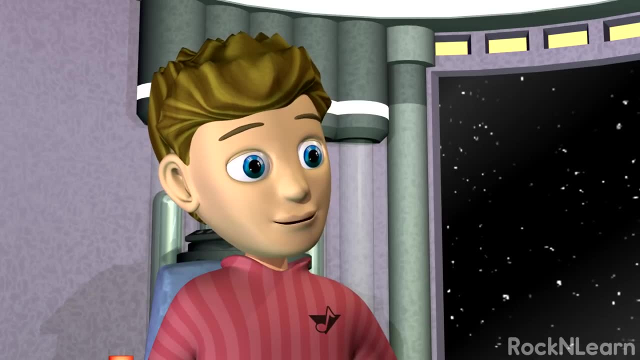 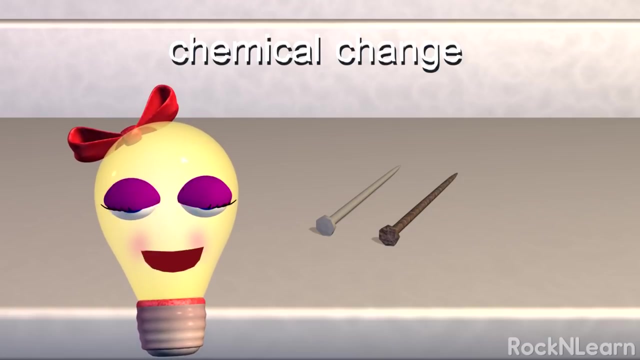 Those are physical changes too. But if you really want to mix things up, you can make a chemical change. Take a look at these nails. This one is all rusty, But how's that different from breaking a stick or crushing a can? Rust is a chemical change. The iron in the nail combines with oxygen in the air to make a new molecule. 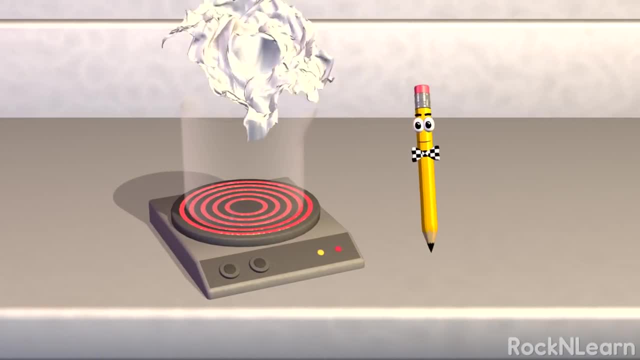 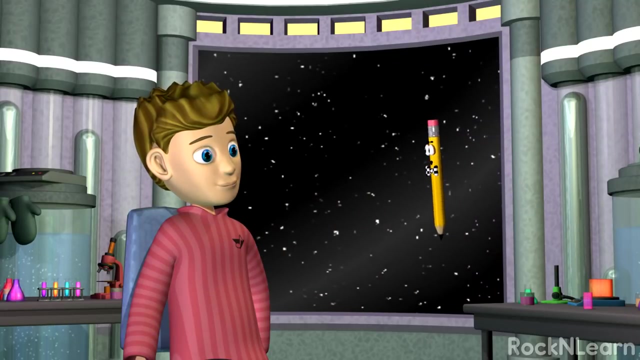 with different properties than iron, And if we burn this paper inside the beaker that will cause a chemical change too. The ashes are different from the paper on the molecular level. We've made a different kind of matter with a chemical change. So far we've learned a lot about pure substances, things that are made of a single element or compound. 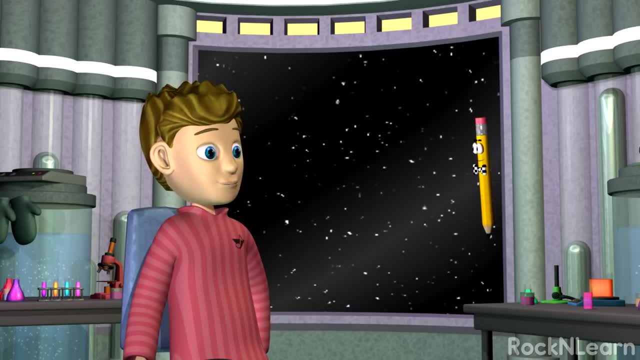 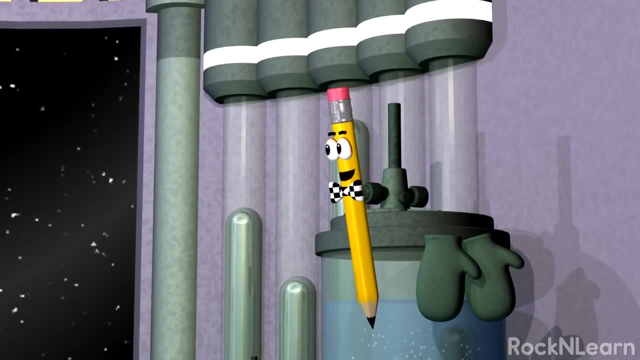 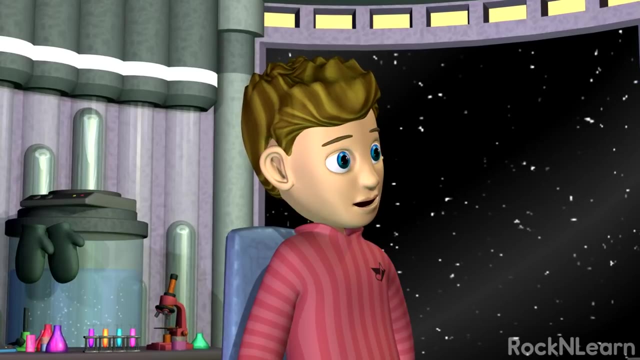 Like helium, It's made of only helium atoms, And water is made up completely of H2O molecules. But some kinds of matter are combinations of different atoms and molecules. We call these things mixtures. But wait, isn't water just a combination of hydrogen and oxygen atoms? 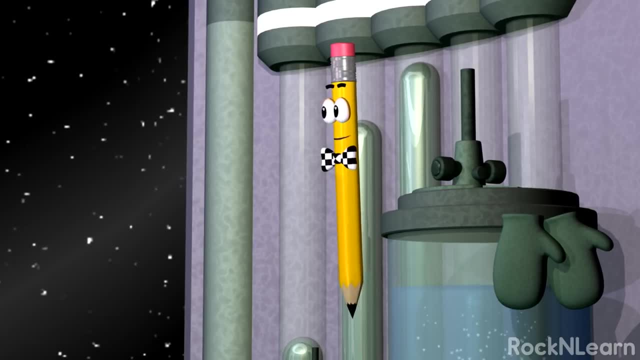 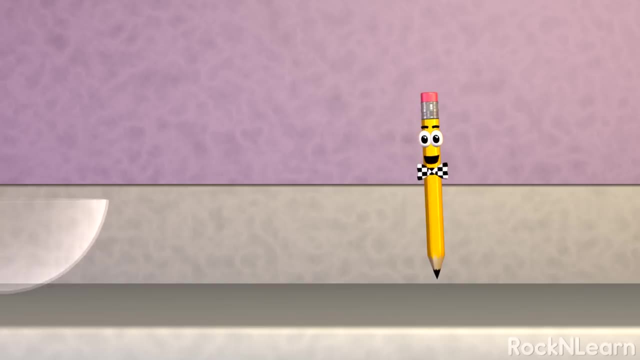 How is a mixture any different from that? With a mixture, you can separate out the parts with a physical change. Let me show you what I mean. Suppose we're making a fruit salad. I like blueberries, strawberries and almonds. We can mix those together to make a salad. 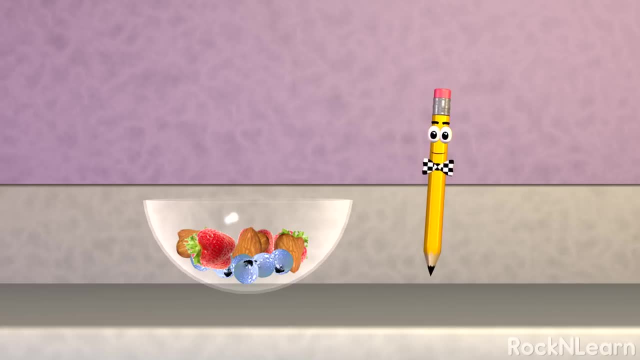 This salad is a mixture. I understand what you're getting at. You could pull out the almonds if you didn't like those. What are you nuts? Just kidding. As I was saying, you can separate the salad back into blueberries, strawberries and almonds. 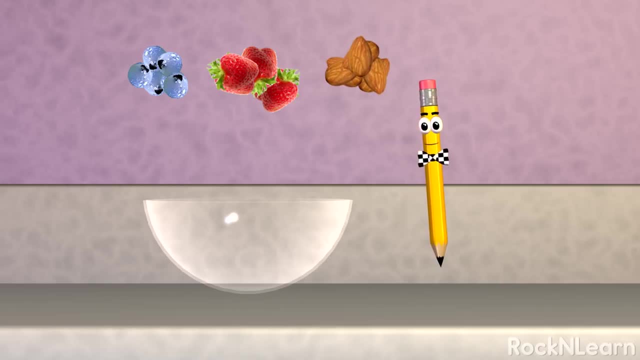 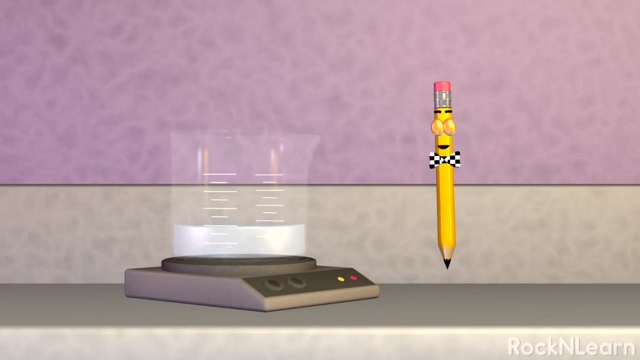 almonds. so the salad is a mixture, But you can't separate water back into hydrogen and oxygen with a physical change. Bravo, Now check this out. Let's pour salt in this beaker of water. Salt and water are each pure substances, but they blend together to make a special